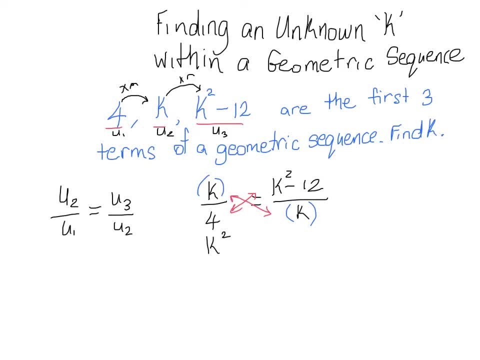 And on the right side we'll have to distribute or 4.. So we have to do 4 minus k, squared minus 12.. So we're distributing that 4, and we get 4k squared minus 48.. Now that square there tells us that this is a quadratic equation. 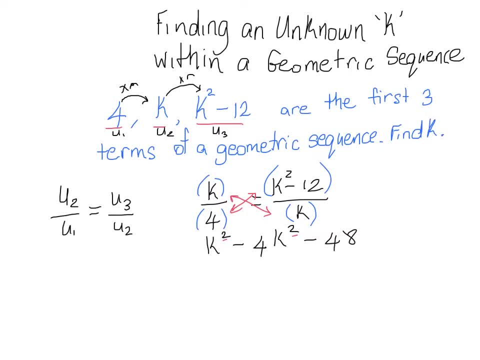 which means that, oh, hold on, we have a little. there we go. which means that, in order to solve a quadratic equation, you want to make it equal to 0 first, So we can take k squared away from both sides. 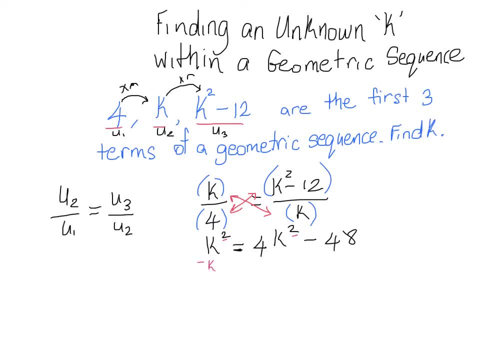 and we'll get- let's see k squared from both And we'll get that 0 is equal to 3k squared minus 48.. So from here there is a common factor of 3, which we can take out, and we get that k squared. 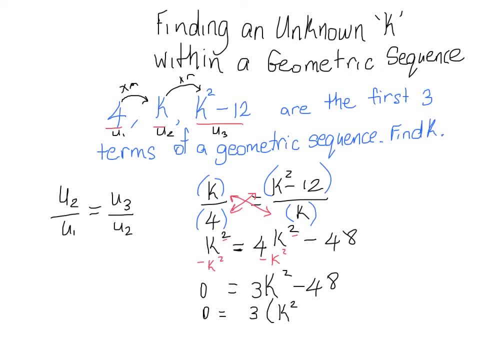 3, sorry, we get 3 times k. squared minus 16 is equal to 0.. From this point, we can now do the difference of two squares, And I'll do it. on this side We have 3 times k. squared minus 16 is 0.. 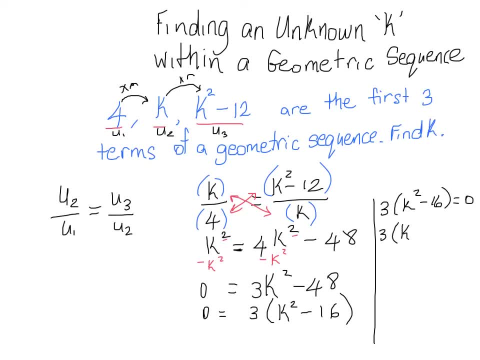 So I can factor this k squared minus 16, and I get 4 on that side, plus positive 4 and negative 4 over here, And that's equal to 0. Which means now we have three numbers being multiplied, we have 3, which cannot be 0.. 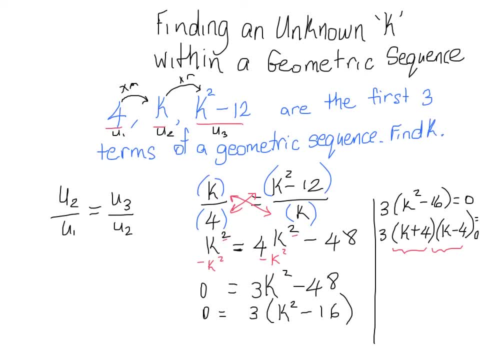 We have k plus 4.. So that could give us that k is negative 4 to make that 0. Or let's rewrite that, or k is 4.. So in order for that to be equal to 0,, k would either have to be negative 4 or 4.. 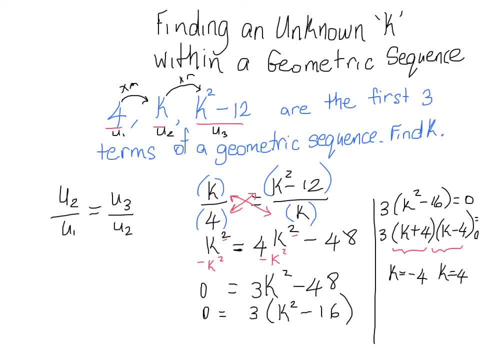 And that's the only way to get that- that equation equal to 0.. Now I wouldn't continue on from this question without checking to make sure that your answers make sense, So let's do that now. Okay, so if k is negative, 4,.